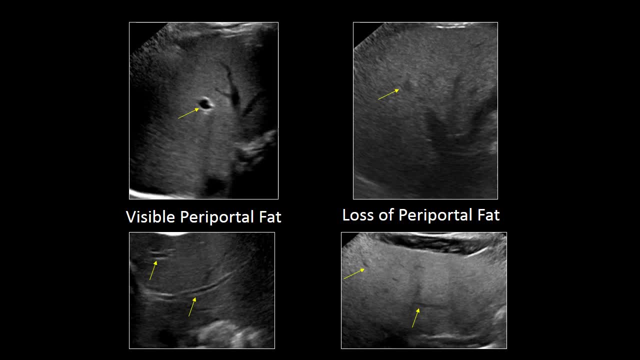 should see the portal veins surrounded by periportal fat. In patients with hepatic steatosis, that rim of hyper echogenicity or rim of fat is no longer visible because the liver has become so fatty that it obscures the periportal fat, And you can see two examples on the right-hand side. 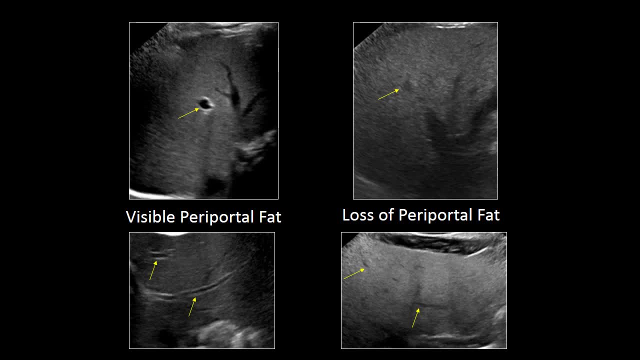 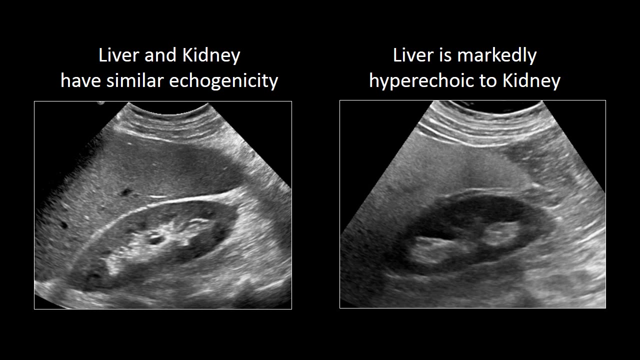 of your screen where arrows point to the portal veins and we do not see that characteristic periportal fat. So we can be very confident that there is hepatic steatosis in both of these cases. We can also use the kidney's echogenicity as an internal reference. 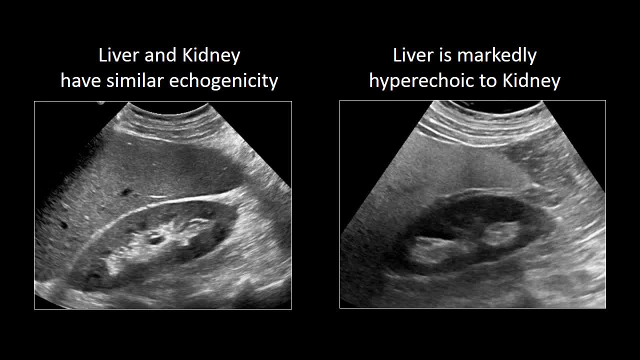 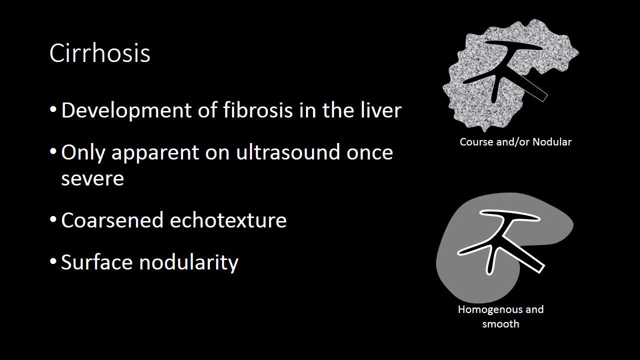 The kidney and liver should have similar echogenicity, or the kidney should just be slightly darker than the liver. When the liver becomes steatotic, it becomes increased in echogenicity and the kidney will appear very dark or hypoechoic relative to the hyper-echoic liver. Now let's 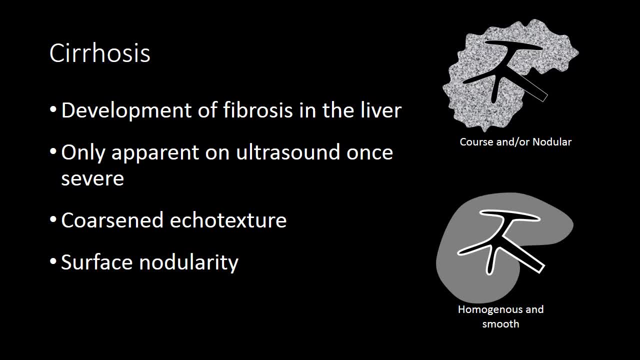 switch gears and look at cirrhosis. Cirrhosis is the development of fibrosis in the liver and oftentimes fibrosis in the liver is only apparent on ultrasound once it becomes very severe or once it is truly developed into cirrhosis and not just early stage fibrosis. We are looking for two. 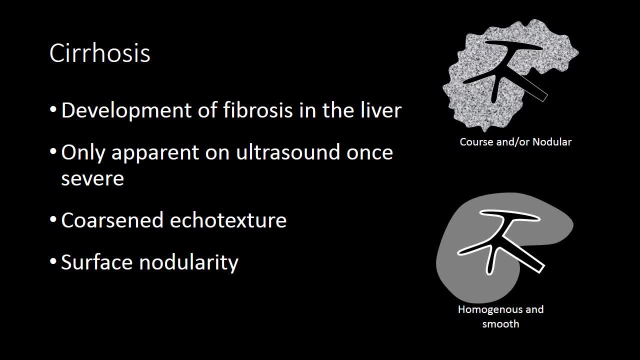 different signs. One: coarsening of the echo texture. So when the liver becomes fibrotic, the fibrosis creates a heterogeneous or coarse appearance to the liver function parenchyma. The other finding we're looking for is surface nodularity. The normal liver should. 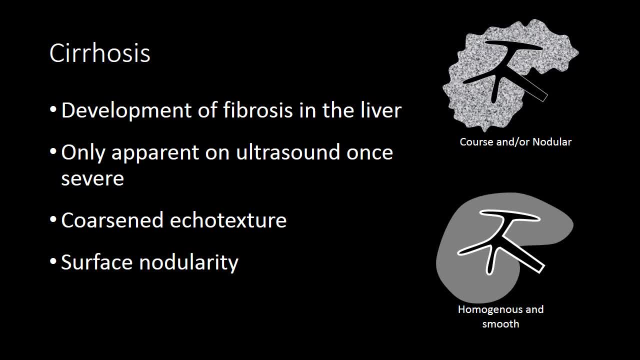 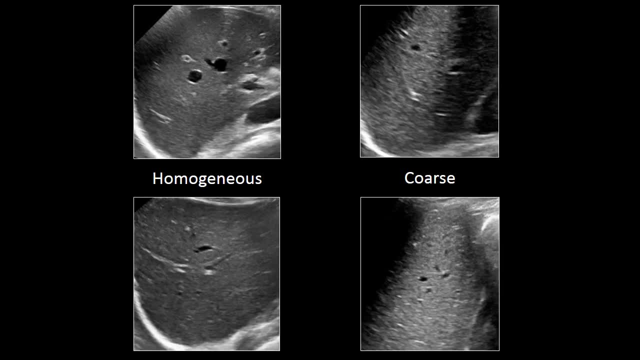 have a nice smooth surface and in the setting of cirrhosis the liver surface will become irregular or nodular. Here are examples from four different patients. On the left-hand side we have two normal livers in which the liver parenchyma is very homogenous. The only areas 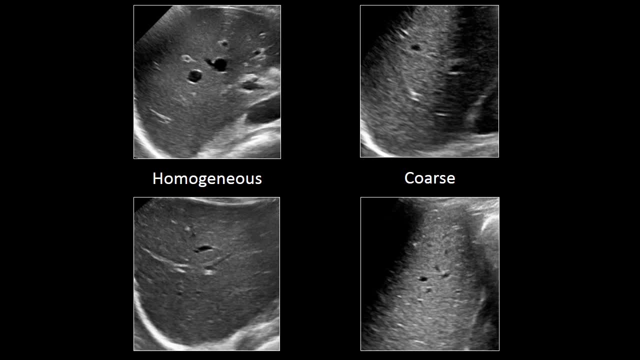 where there is texture to the liver are where the vessels are and those vessels provide normal texture. but the actual tissue of the liver is very smooth and homogenous. On the right-hand side of your screen you can see examples of two livers with cirrhosis and unlike the livers on, 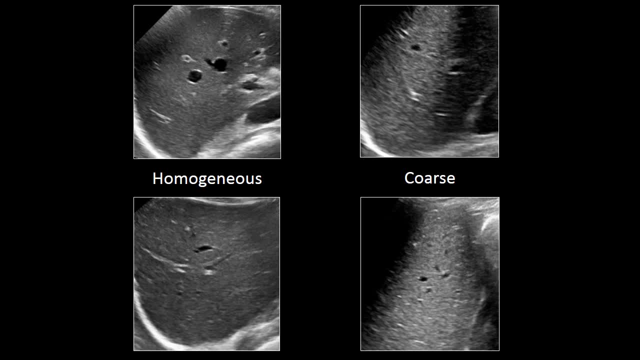 the left, the livers on the right have more texture to them and they're more coarse, and that coarse appearance is due to the fibrosis within the liver. There is a wide spectrum of normal and abnormal and I think that being able to detect a coarse 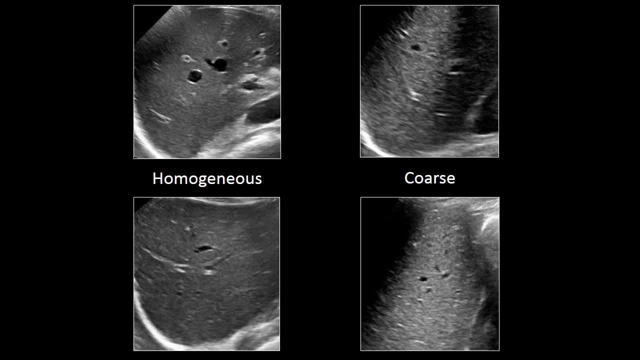 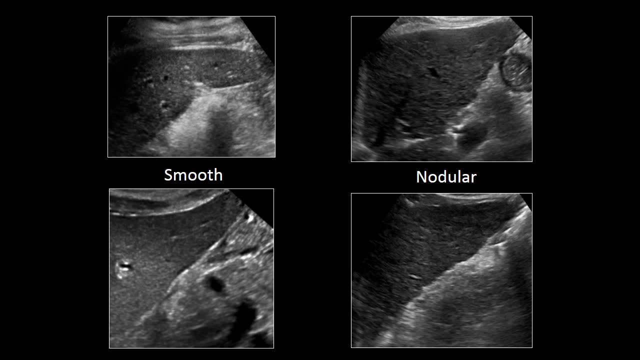 liver- unless it's an extremely coarse liver- can be difficult. One thing that you can rely on with more certainty, however, is nodularity of the liver surface. A normal liver should have a very smooth surface. On the right-hand side of your screen you have 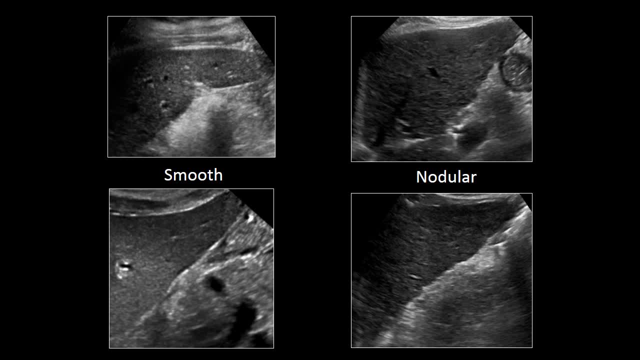 examples from two patients with coarsened livers but also nodular liver surfaces, and I highlight that nodularity, with a line here and a line here, and now I'll remove the line and let you look back at those livers and you can see the sort of undulating contour of the liver and you can 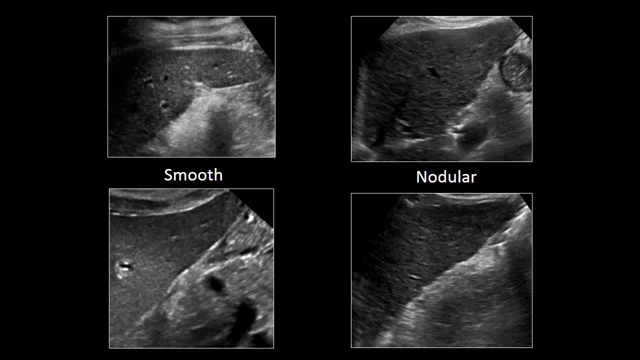 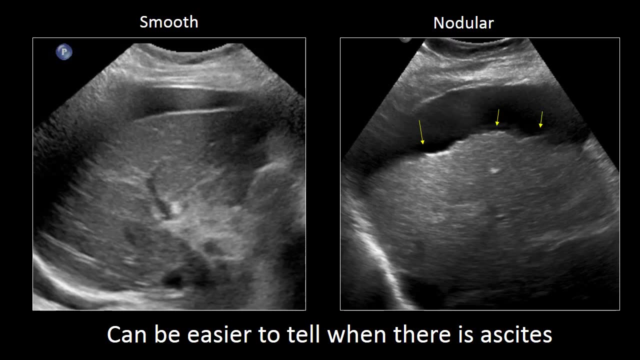 compare that to the two examples on the left-hand side of your screen which have a nice smooth liver surface. When ascites is present, oftentimes nodularity is accentuated. I've presented two cases. One person on the left has ascites but does not have cirrhosis, and you can see that nice smooth contour to the. 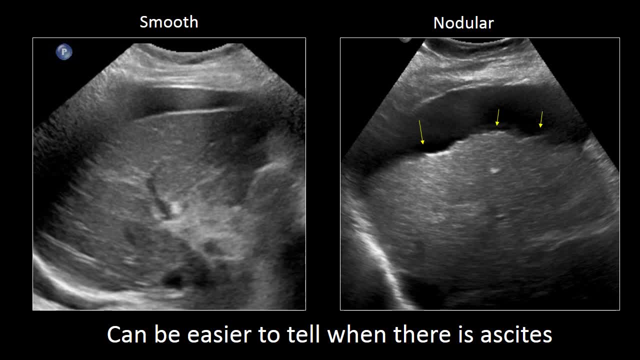 liver and you compare that to the person on the right who has ascites and a very irregular or nodular liver, and when we see this nodularity we can have a high degree of confidence in the liver and we can see the difference that the patient has underlying cirrhosis. 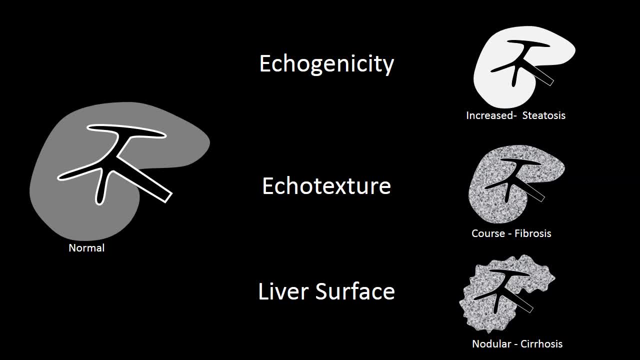 So a normal liver should have a homogenous tissue or homogenous liver parenchyma and it should be similar in echogenicity to the kidney and you should be able to see distinct rims of periportal fat along the portal veins. When there is steatosis, the echogenicity of the liver increases relative to the 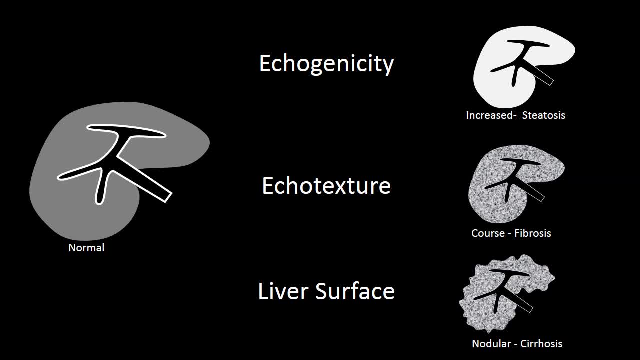 kidney and we lose the distinct rim of periportal fat. As fibrosis develops, the liver parenchyma gets coarse or more heterogeneous, and then, once cirrhosis has developed, we can often detect nodularity to the liver surface, giving us a high degree of confidence. 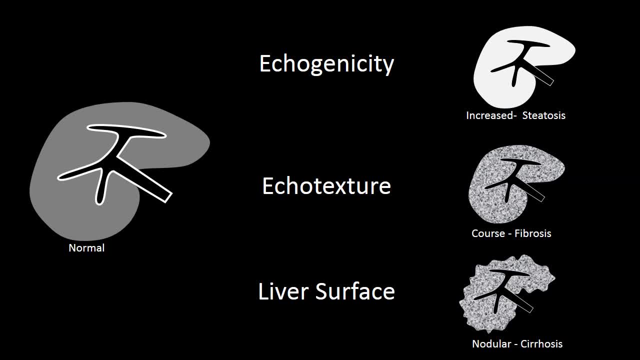 of underlying liver fibrosis and cirrhosis.